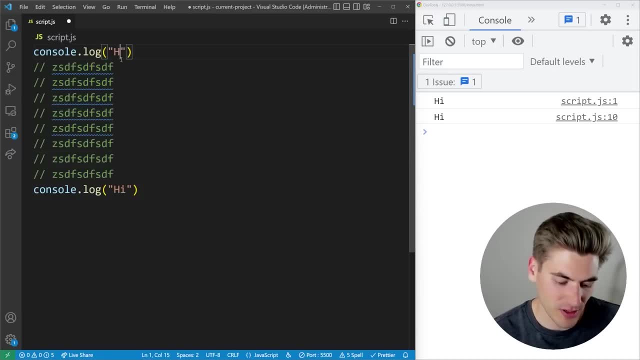 But what happens if I want to change this console log high to say hello. Well, I need to change it to hello here. Okay, now I need to change it to hello down here. So I had to change my code in two different places. Essentially, I know for a fact that 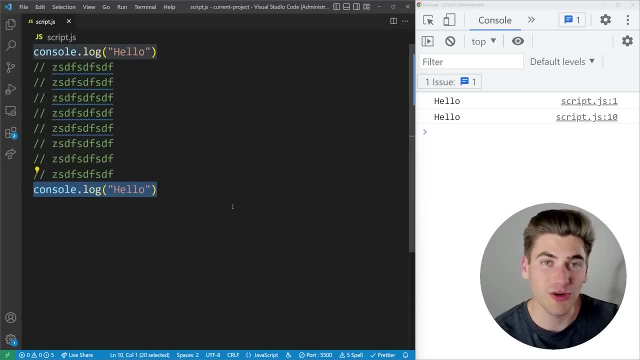 this console log that says hello and this one on the bottom are always going to be exactly the same, And I want them to do the exact same thing every single time I call them. But right now they're copied between different places And every time I change one I need to make sure I 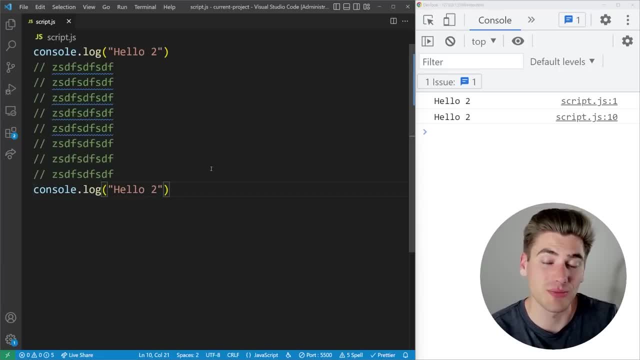 update the other one. This is the perfect use case for a function because a function in JavaScript? all it does is it takes some type of logic, So console logging hello to, and it just puts that inside of a particular piece of code that you can run whenever you want And it's always going to do. 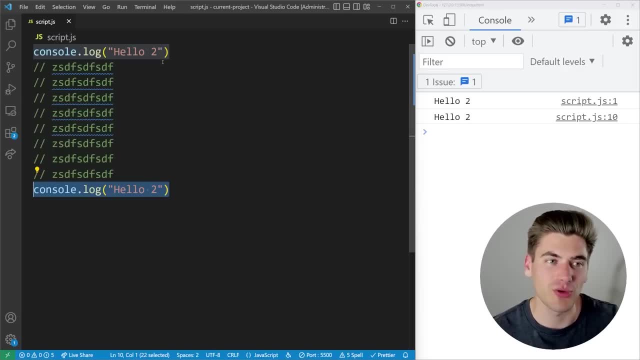 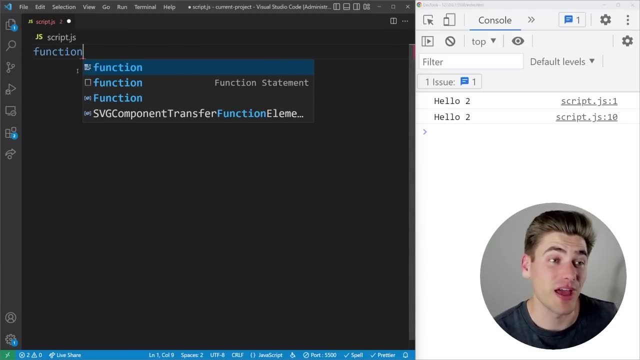 the same thing every single time. So let me show you really quickly how you would create a function to do this little bit of a log. So to create a function, you just need to type the keyword function And you'll know you've done this correctly. if in your editor it'll probably. 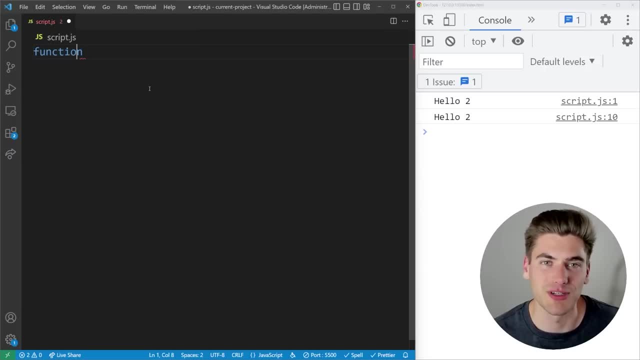 turn a different color- In my example it turns blue, but it could be any color for your particular editor- then you need to give your function a name. So just hit space, give it a name, we'll call this one. say hi. Now the final step you need to do is you need to close this off with. 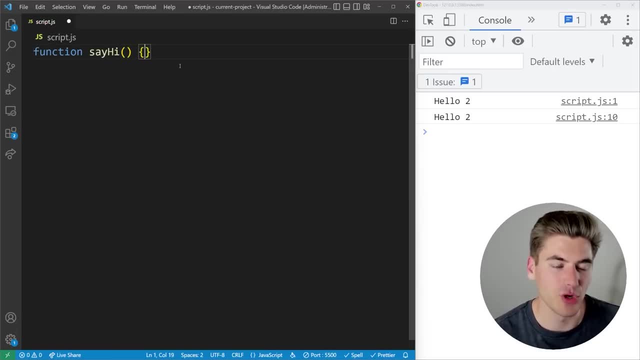 parentheses. So you put an open and a closing parentheses And then finally some open and closing curly braces. So what we have here again is we have the keyword function, we have a name for a function, And then functions can actually take arguments and parameters inside of them. So 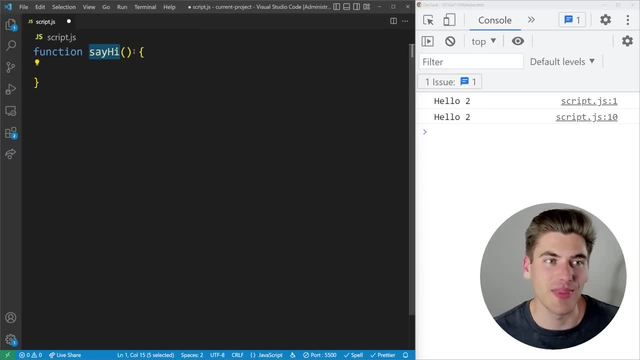 you can like pass code to a function. In our case we're not dealing with that, And that's why our parentheses here are completely blank, And for now that's perfectly okay. Then the final thing we have is these open and closing curly braces. everything between these curly braces is going. 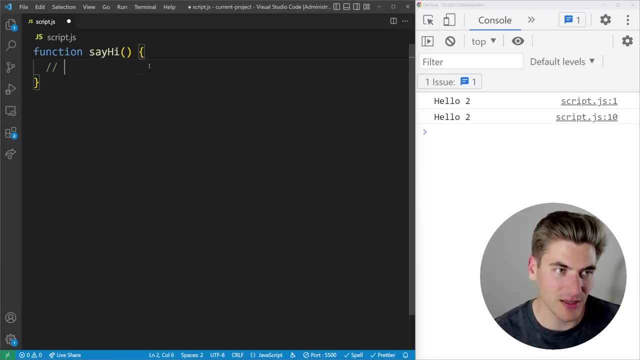 to be the code that gets executed in your function. So everything we put inside of here, all of this gets executed every time we call our say hi function. What I'm going to do in here is I'm just going to console log Hi And if I save my code, you'll notice nothing gets printed on. 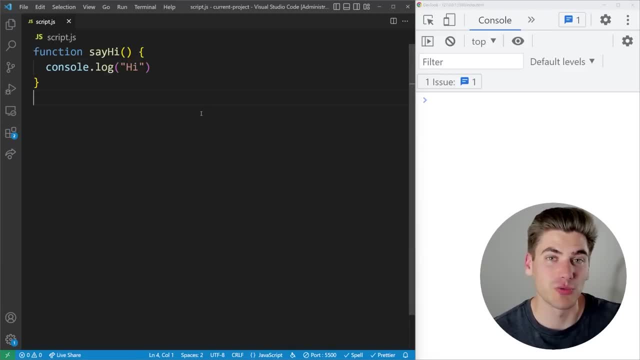 the right hand side of my screen, But we also have no errors at all. So this code is working, but it's not doing anything. And that's because, by default, when you create a function, which is done here, the function just stores some code to execute later. it doesn't do anything, it doesn't. 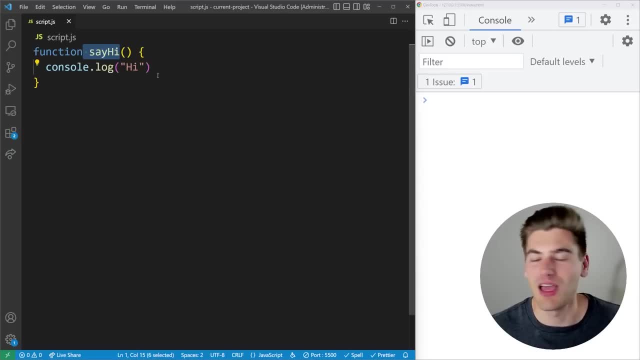 run any code. it's just saying, hey, I have this function called, say hi, And when you call it I'm going to run all the code inside these curly brackets, But for now I'm not going to do anything until you tell me to do something. So let's talk about how we actually call a function. To call a. 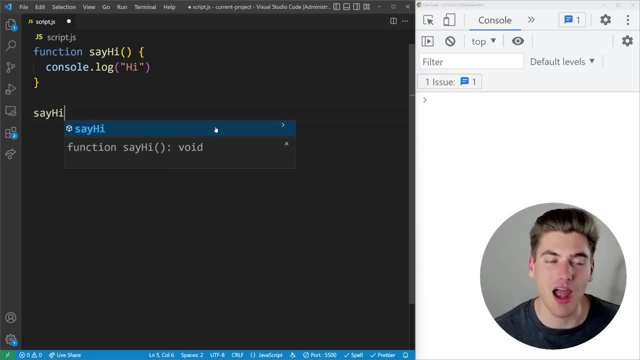 function. all you do is you type out the name of the function, in our case say hi- and then you again use parentheses. So open and close the parentheses. that's how you tell your function you want to call it. So we're saying: call the say hi function and pass absolutely nothing to it. 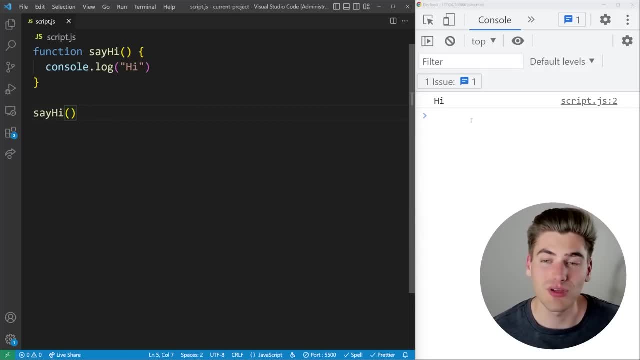 and put anything inside of our parentheses here. Now, if I run this, you can see it prints out hi, because what's happening is it creates our function right here, then later in our code we're calling that function, And when you call the function it just goes into these curly brackets. 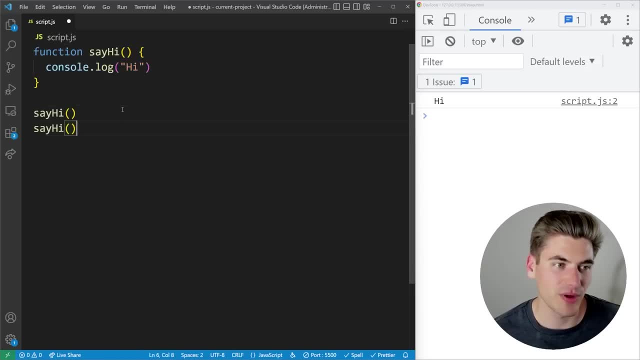 and runs all the code inside of them And that's all that happens. If we run this function a second time, you'll see it prints out hi twice And if I change this to hello, I only have to change it in one place and updates both of the functions that are being called. That's again one of the huge 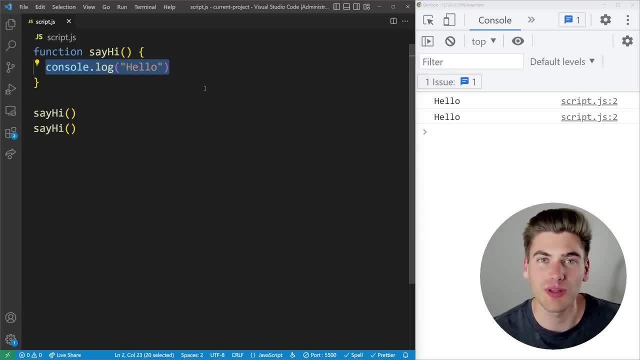 benefits for functions because you can take logic and code that you're using all over the place, put it in one place and then you can reuse it and change it easily, all in one place. Now, up until this point, all we've done is create a very basic function that doesn't take any arguments and just 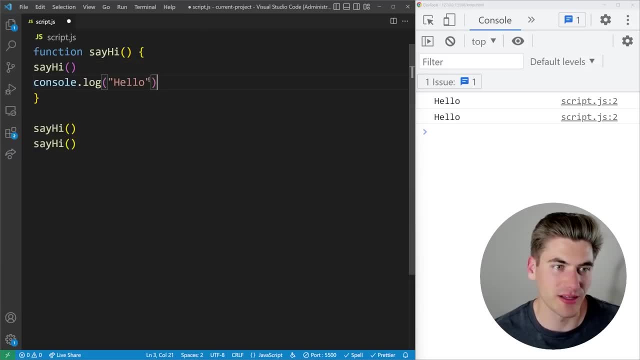 does whatever we tell it to. We can, if we want, make this have multiple lines, So this could say hello and bye, And now you can see when we call this it's going to say hello and then it's going to say bye. So you can have as many lines of code as you want in here, as long as they're. 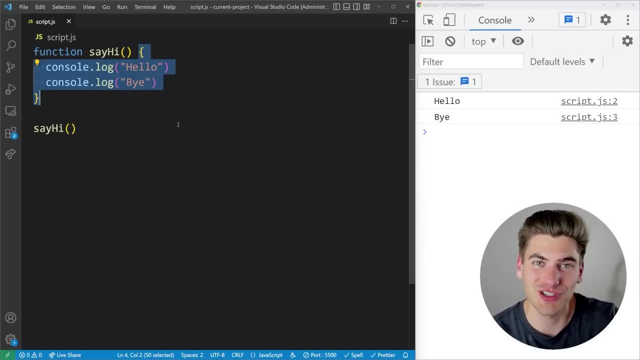 between these curly braces. What happens if you want to pass code to a function. Let's, in our case, try to create a sum function. So we're going to say the function and we're going to call it sum. We're going to do those opening and closing parentheses and opening. 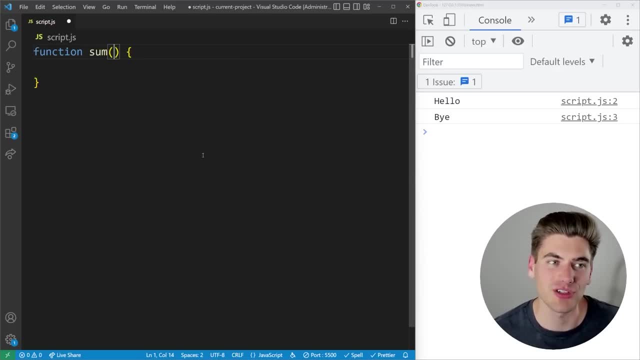 and closing curly brackets. But I want to pass some code to our sum function. All you need to do is just give it a name, whatever you want. You can call it anything you want. In our case we'll call it A and we'll call it B, because we want to add the numbers A and B together. 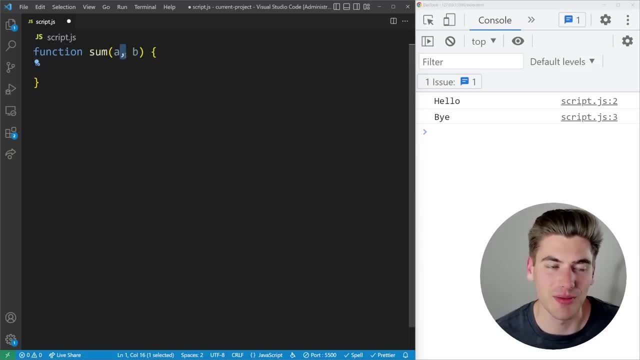 When you pass different variables inside of a function like this, you just need to separate them by a comma. That's all it takes. You don't even need this space. I just put it for readability purposes. And now we're passing in a variable called A and a variable called B. 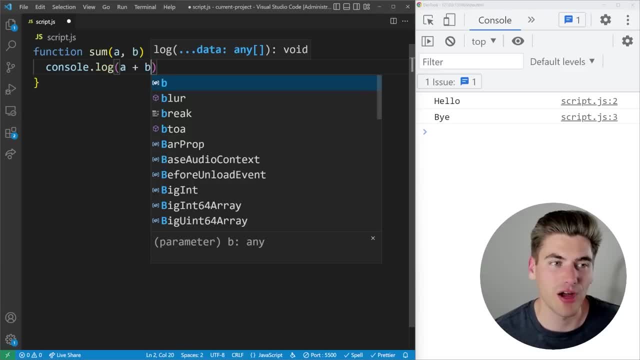 And I just want to log out those two variables together. So I'm just going to log out whatever A plus B is And you'll notice, before I added A plus B these were kind of dark gray color in my editor, And when I add A plus B, 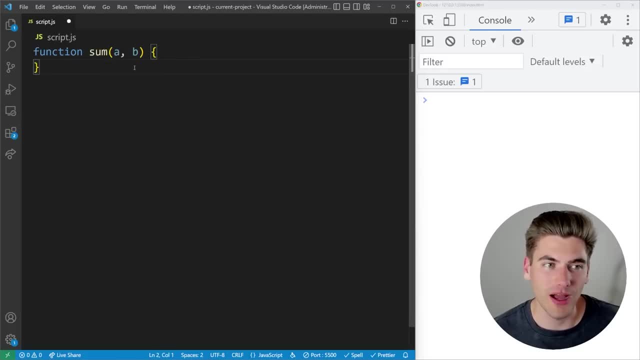 they become a more bright color. That's just my editor telling me that before I wasn't using these variables and now I am using these variables. So now to call this function we just type sum and we put the opening and closing brackets here. opening and closing. 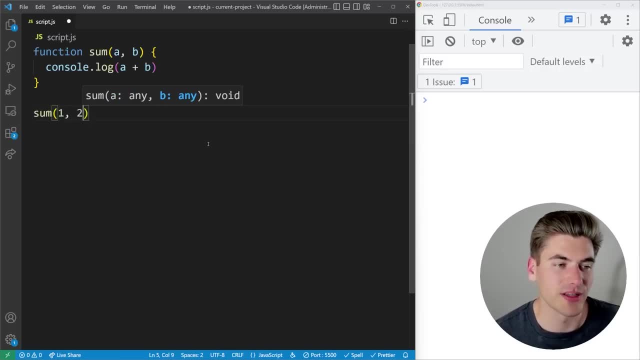 parentheses. But now we also need to pass it a value. So let's pass it the values one and two, again separated by a comma. If I save, you can see it logs out three, because it's just adding one and two, which is what I put in there. So I'm going to call it sum and I'm going to 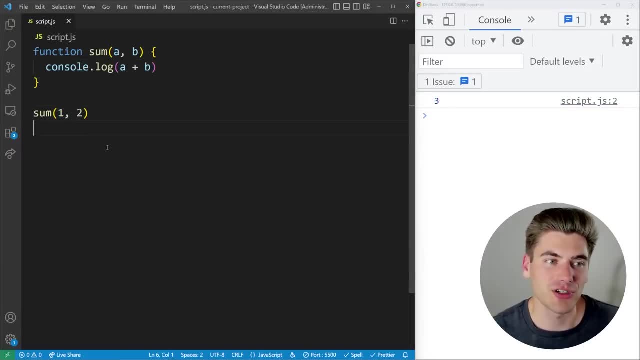 pass into here. So when you have parameters and arguments inside of a function that you can pass between them, you'll notice that whatever the first thing you pass to the function is is just defined as this first variable here. So that is A. You can see if I consolelog A. 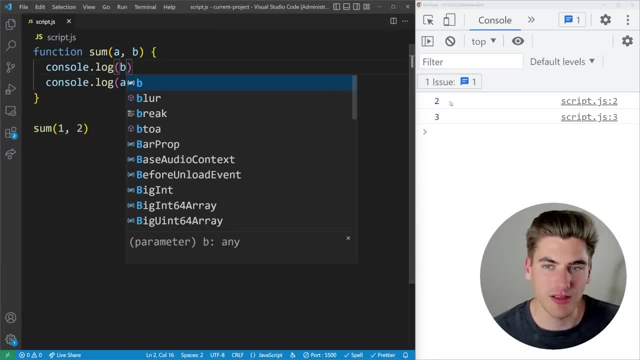 and I save this, you can see it prints out one. If I change this to consolelog B, you can see it prints out two, because whatever your second value is here corresponds to the second value here. So they directly map to each other, one to one, into wherever they're going. 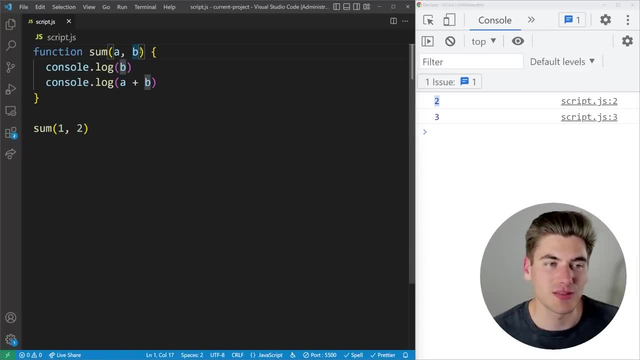 So whatever you put here gets put into this variable. whatever you put here gets put into this variable. So that's what I'm going to do here. So I'm going to go ahead and type variable B here. It's almost exactly the same thing as if you just said: like const A equals one. 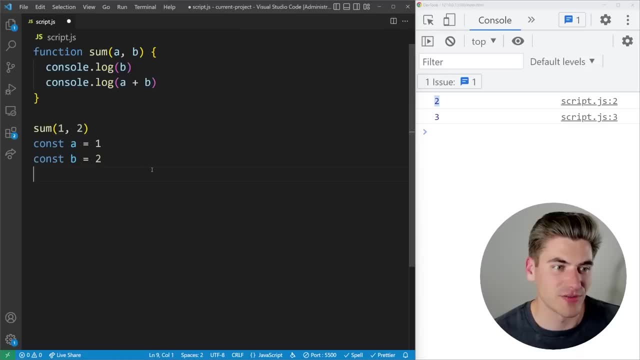 const B equals two, and then you copy whatever code is inside this function and paste it down below. That's the exact same thing that happens when we run sum one and two. So let's get rid of all that code. bring it back to what we had here. Now, what happens, though, if we don't pass a? 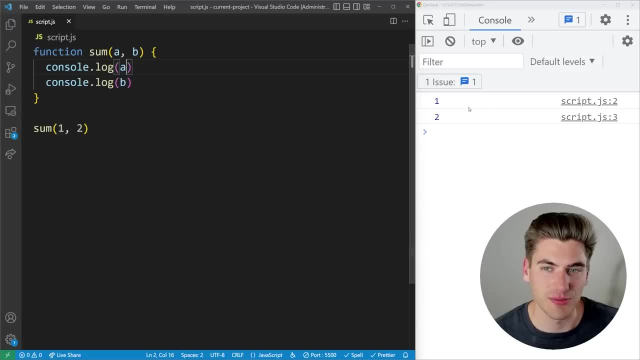 variable for B. So I'm just going to consolelog A and B So you can see it prints out one and two. What happens if I don't pass anything for our second value? If I save, you notice it prints out undefined and it doesn't actually throw any errors. JavaScript is a bit unique when it comes. 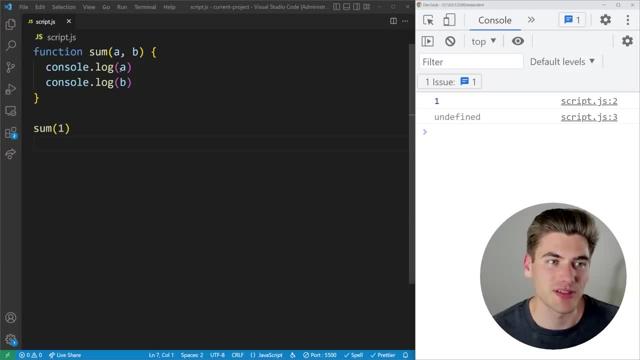 to functions and that it doesn't throw any errors if you don't pass enough arguments. It just sets all the arguments you don't pass to undefined. So if I pass nothing, you'll notice both A and B are set to undefined because I didn't pass anything at all for them. So anytime you leave off some, 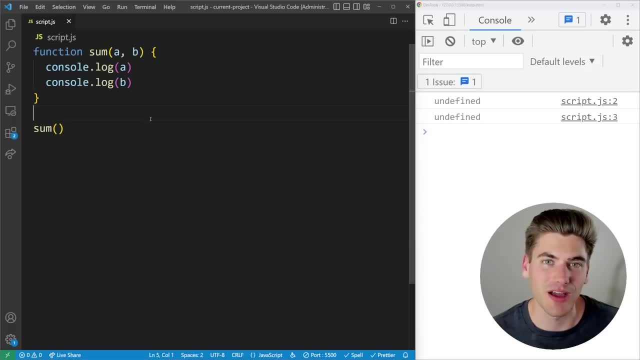 variables that you're trying to pass to your function, it'll always just set them to undefined, So it's really important to understand. Now, the final thing I want to talk about with functions is how you actually get data out of a function, Because up until this point, all we've been doing 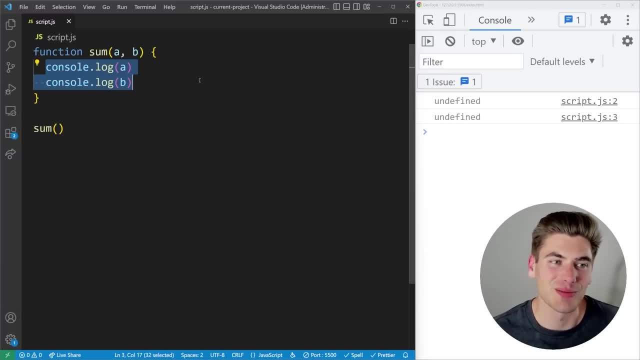 is logging out some information to the screen, but we haven't been returning any data to be used. So instead of just logging out A plus B, I want to return A plus B so I can use it later, And to do that you use the return keyword. So you just type in the return keyword. If you've done it correctly. 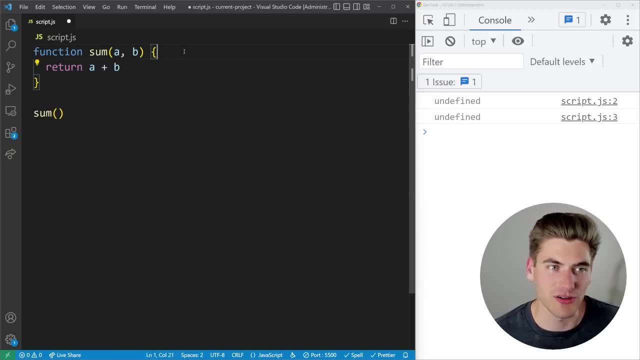 it'll turn a color in your editor and then you just pass whatever you want to return. So I could just say here sum equals A plus B, and then I can return our sum down here and that's going to work just fine. Or I can have what I had before, where it's just inline A plus B, So now whatever A plus. 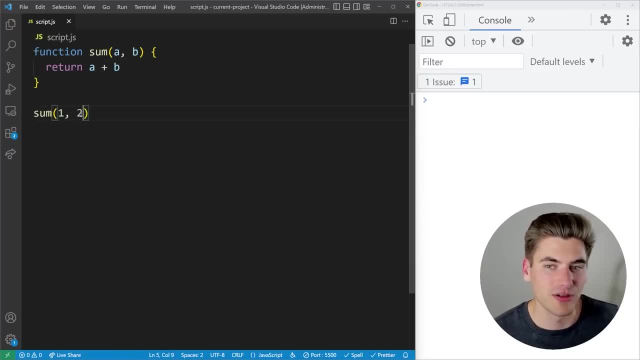 is going to be returned from my function. So again, let's pass in one and two, And when we save, you notice nothing's logged out, which is great, But our sum is being printed out here. So we have our actual sum value, which is right here. we'll just call it value, make it a little bit. 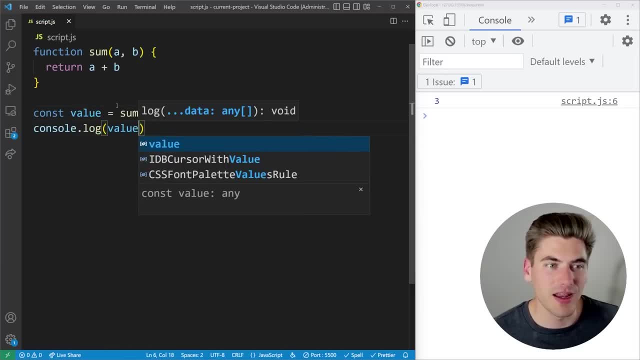 easier to read And I can consolelog our value And now you'll notice it prints out three. So when you use the return keyword, what essentially happens is it takes whatever that value is you're returning and it puts it inside the variable of that function. So it just comes. 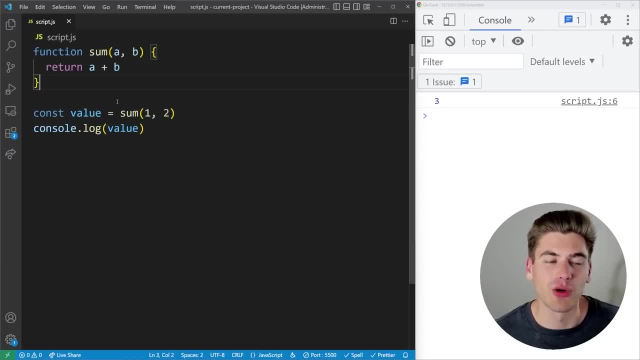 out of the function. This is really powerful And one of the main use cases for a function is getting some other data from that function. it's going to do a bunch of stuff and then spit out some data for you. So all the time you're going to see code like this where you set a 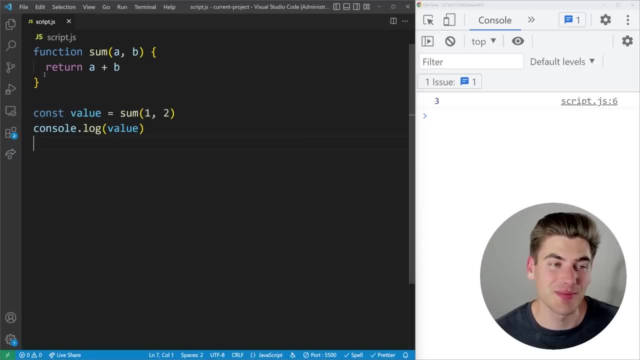 value based on the result of a specific function. Another interesting thing about this return keyword is it makes sure no code runs after it. So we just say consolelog never will run And we save. you'll notice this never gets printed out. it's even kind of grayed out inside of my editor. 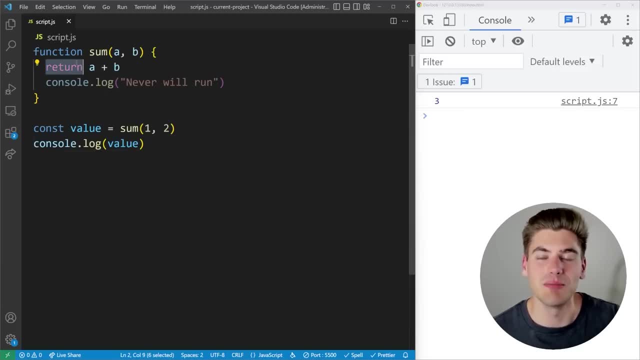 And that's because every single time, whenever you run return, the function immediately exits out. nothing else afterwards is ever going to happen, So that's one of the things that we want to be run. This is actually really useful And people will use this to exit out of functions early. 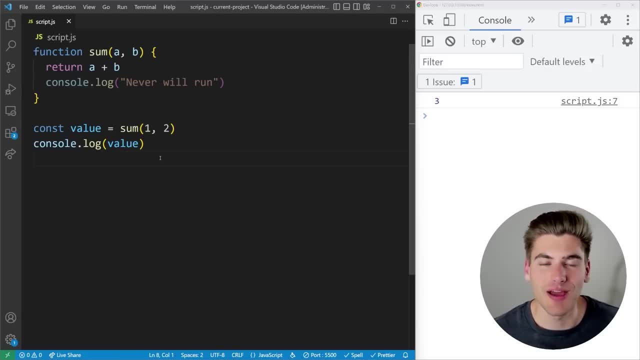 if there's like an error of some form. Now, something really neat that you may have actually picked up on this video is that consolelog is actually a function on its own. we just change this back here to high. you'll notice that this works just like a normal function. we're calling: 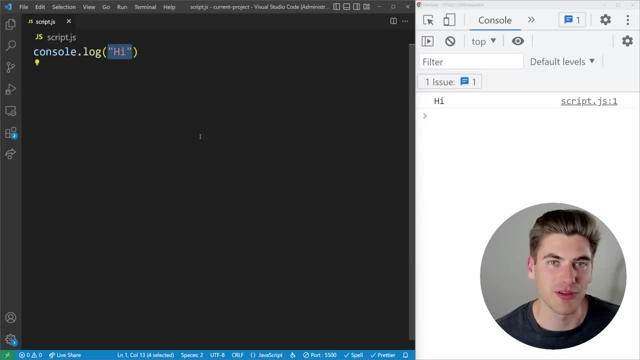 this log function with our parentheses and we're passing it a specific value. And consolelog is really cool because that's what it is. it's just a function that takes in some values, And there's lots of functions built into JavaScript that you've probably already used before, But this is. 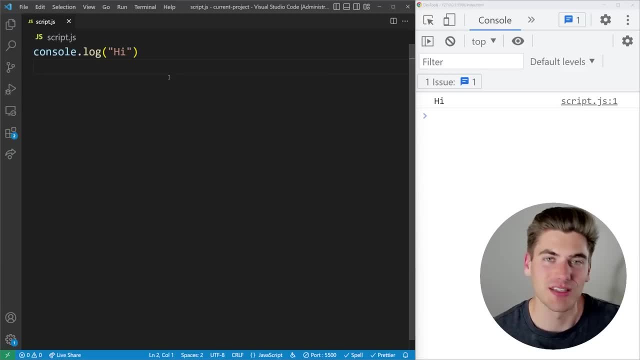 probably the one you've used the most, And you may not have even realized that this itself is a specific function. So that's why it's really important in JavaScript to make sure you understand the fundamentals of what is going on, Because if you do, it makes all these magical. 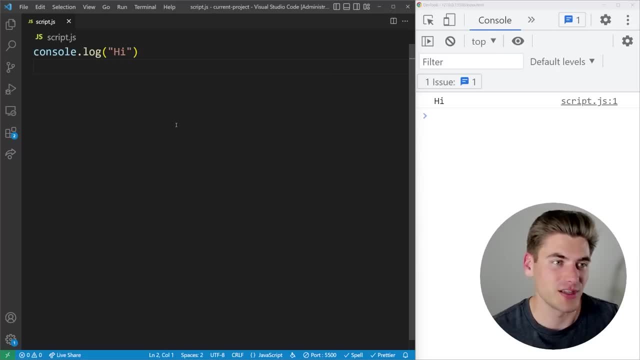 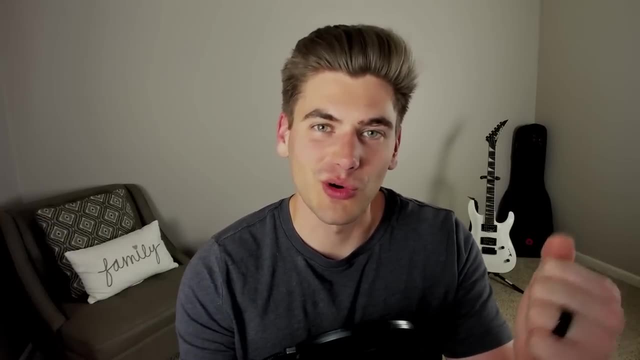 seeming things like consolelog much simpler to understand because it really is just a function, that's all it is. So if you're interested in actually learning those building blocks of JavaScript and making sure you understand the core concepts so that you can really truly,